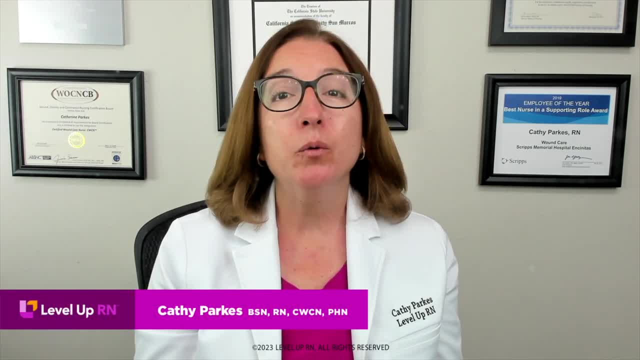 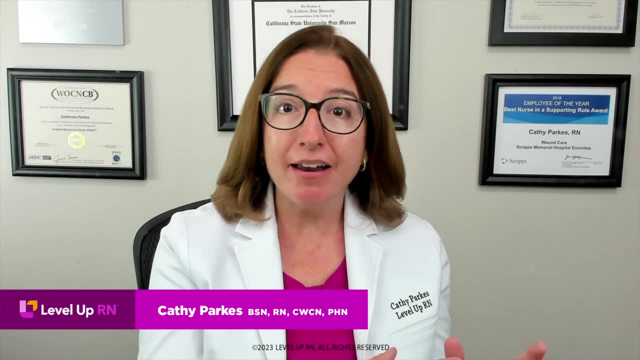 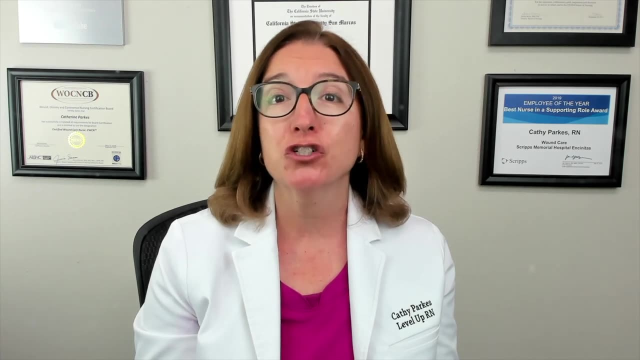 Hi, this is Kathy with Level Up RN. In this video I will explain how to do temperature conversions, So I will provide the formulas for converting from Fahrenheit to Celsius, as well as Celsius to Fahrenheit, And then I will work through a couple of temperature conversion problems. 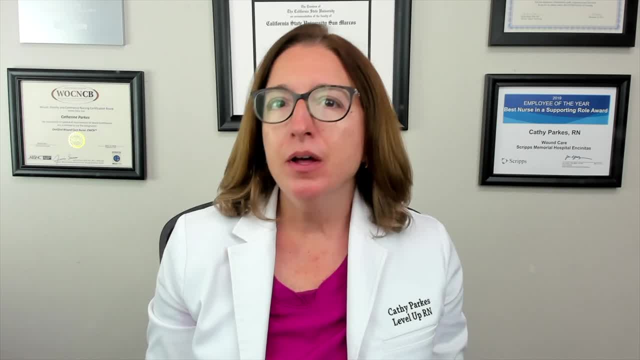 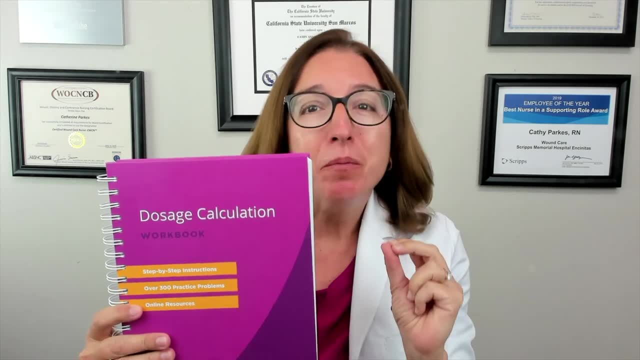 You can find all the information that I'll be covering in this video in our Level Up RN dosage calculation workbook. If you are in nursing school, then you know how important it is to master dosage calculations, And our workbook will help you do just that. 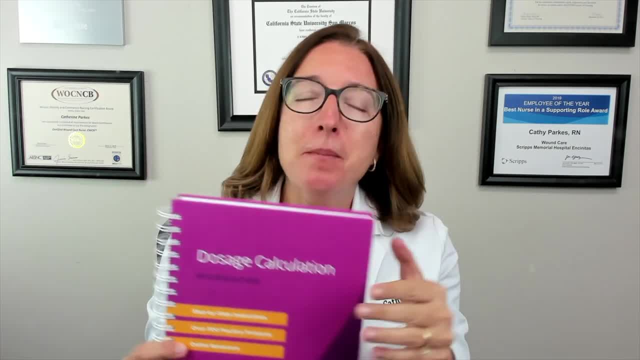 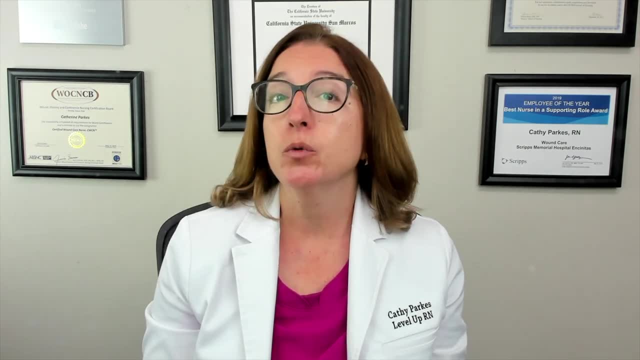 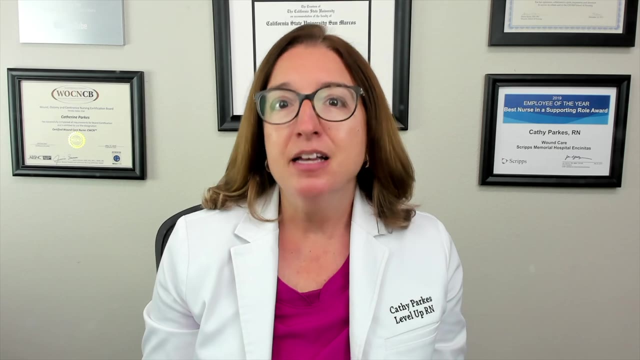 For more information about our workbook, you can click here. But in a nutshell, our workbook contains all different types of dosage calculation problems that you are likely to encounter in nursing school, And we demonstrate how to solve each problem using multiple methods, so you can. 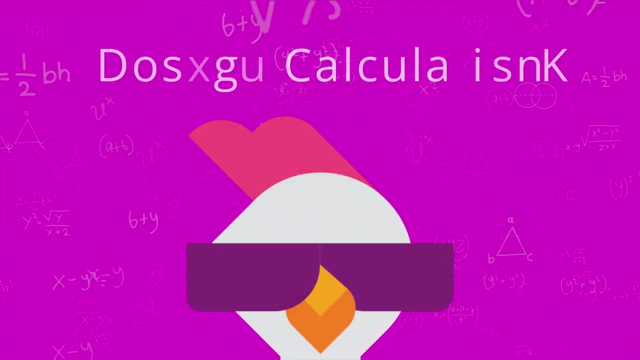 pick the way you want to do it, And if you have any questions, feel free to reach out to me. Thanks for watching. I'll see you next time, Bye-bye, All right, In this video I am going to work through some temperature. 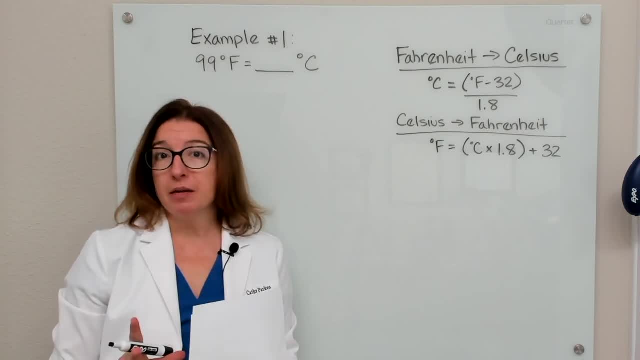 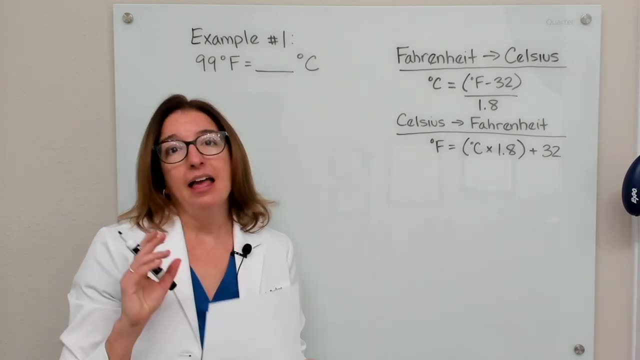 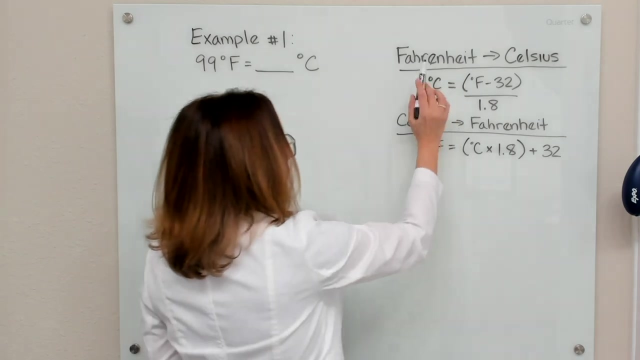 conversion problems. So we are going to work through an example problem where we go from Fahrenheit to Celsius and another where we go from Celsius to Fahrenheit, And in order to do these types of problems, you definitely have to memorize these equations over here. So when we're going from Fahrenheit to Celsius, this is the equation you want to use You. 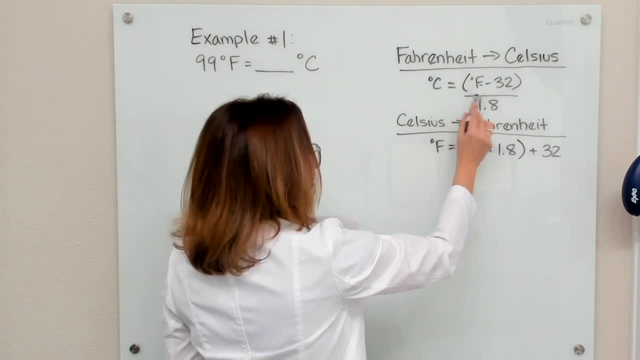 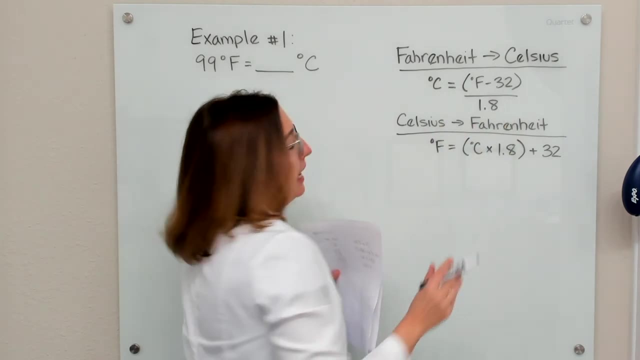 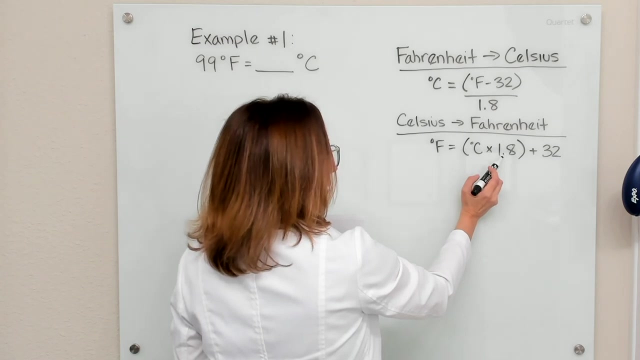 want to take your temperature in Fahrenheit, subtract 32, and calculate that, and then take that answer and divide by 1.8.. And then, when we're going from Celsius to Fahrenheit, you want to take the temperature in Celsius, multiply times 1.8, and then take the answer to that and add 32.. 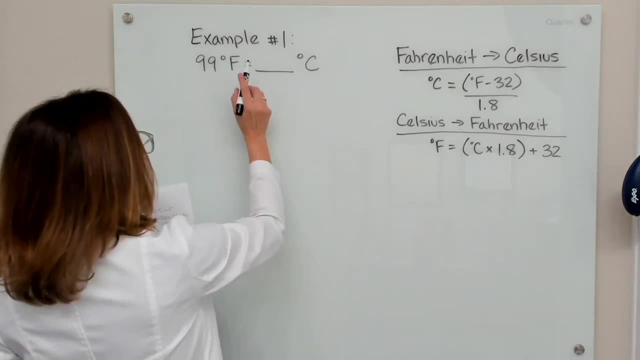 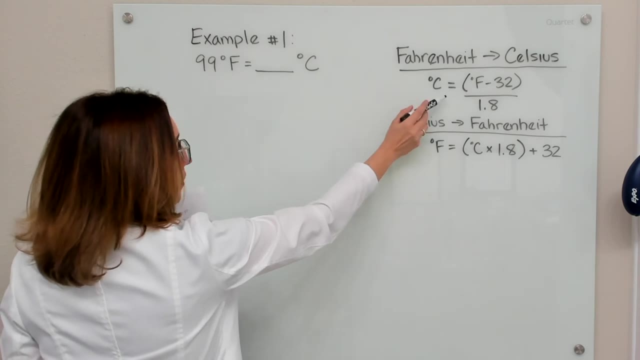 So let's work through our first example problem here. With this problem, we have 99 degrees Fahrenheit and we want to take the temperature in Fahrenheit, multiply times 1.8, and then take the answer to Celsius. So we're going to be using this equation here. So the degrees Celsius equals.